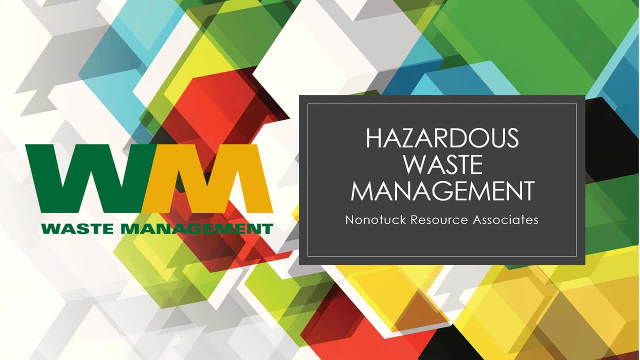 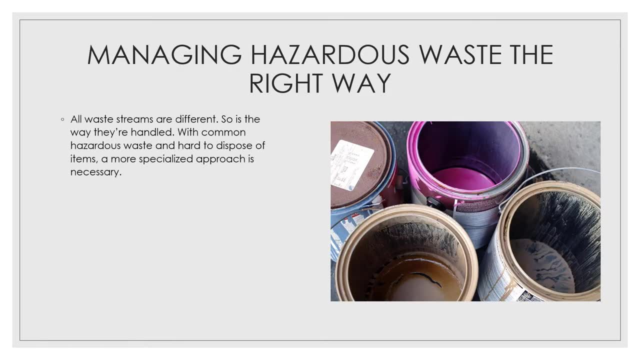 Hazardous Waste Management from Nonotuck Resource Associates: Managing hazardous waste the right way. All waste streams are different. So is the way they're handled. With common hazardous waste and hard to dispose of items, a more specialized approach is necessary Due to safety concerns. not all items can be collected with your normal trash pickup. 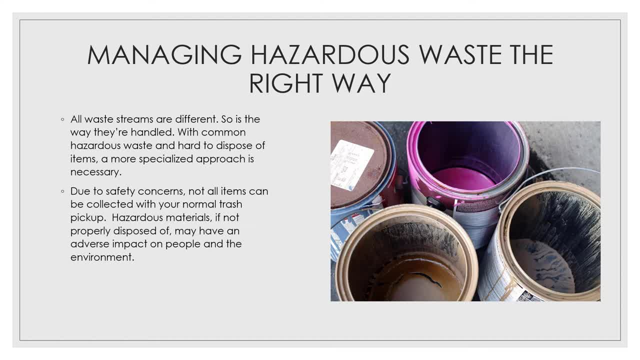 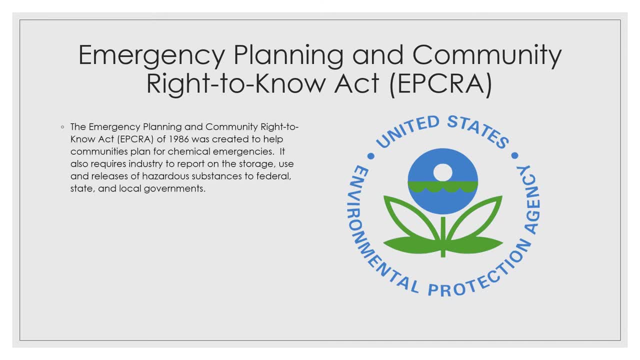 Hazardous materials, if not properly disposed of, may have an adverse impact on people and the environment. Emergency Planning and Community Right to Know Act. The Emergency Planning and Community Right to Know Act of 1986 was created to help communities plan for chemical emergencies. 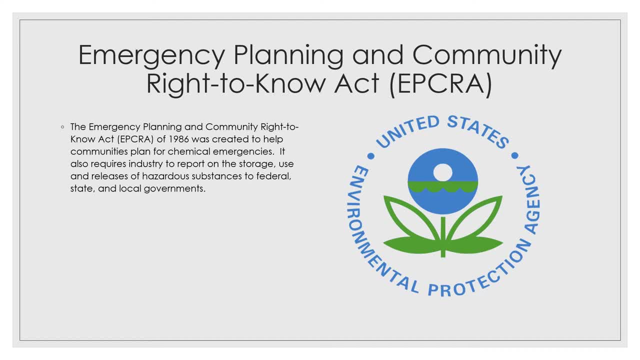 It also requires industry to report on the storage, use and releases of hazardous substances to federal, state and local governments. EPCRA requires state and local governments and Indian tribes to use this information to prepare for and protect their communities from potential risks. 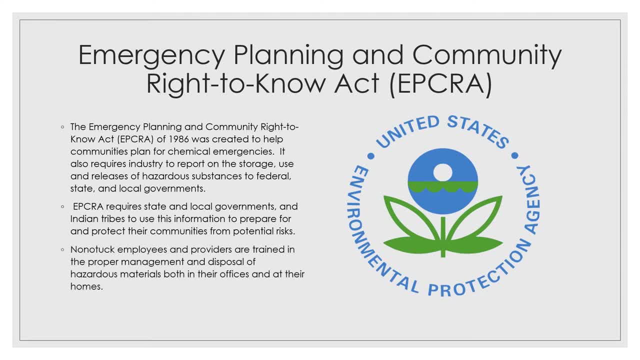 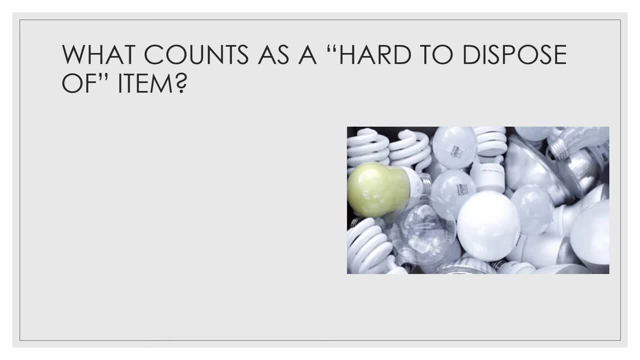 Nonotuck employees and providers are trained in the proper management and disposal of hazardous materials, both in their offices and at their homes. What counts as a hard to dispose of item? Below is a list of common hazardous materials that can be collected through the At Your Door service. 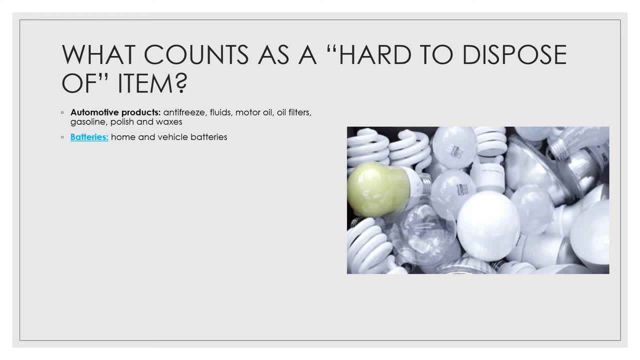 Automotive products, such as antifreeze fluids, motor oil, oil filters, gasoline polish and waxes. Batteries, such as home and vehicle batteries. Electronics, including TVs, computers, laptops, cell phones, printers, fax machines, MP3 players. 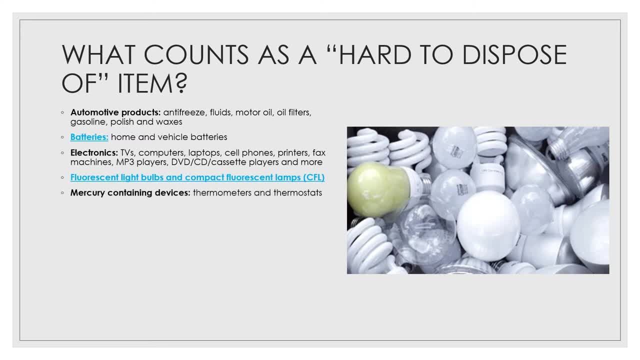 DVD, CD and cassette players and more. Fluorescent light bulbs and compact fluorescent lamps. Mercury-containing devices such as thermometers and thermostats. Paint products, including oil-based latex and spray paints. caulking wood preservatives and wood stain. Guarding chemicals like pesticides, herbicides, fertilizer and insecticides. 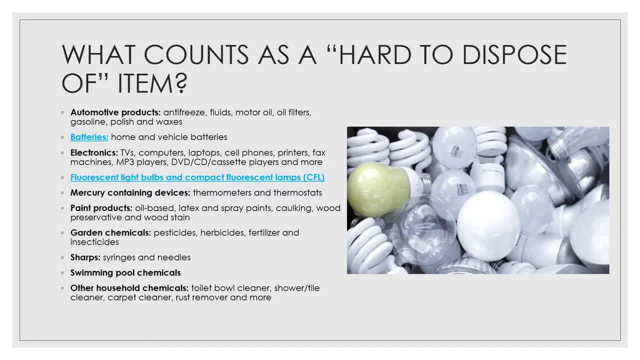 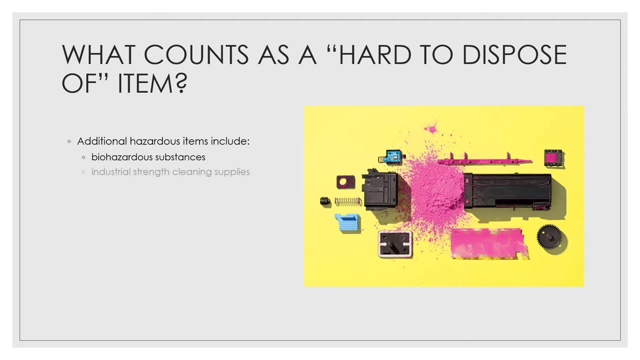 Sharps like syringes and needles, Swimming pool chemicals And other household chemicals like toilet bowl cleaners, shower and tile cleaners, carpet cleaners, rust remover and more. Additional hazardous items include biohazardous substances, industrial strength cleaning supplies, oil-based paints, copier, toner and computer monitors. Handling and storage- Nonotuck. 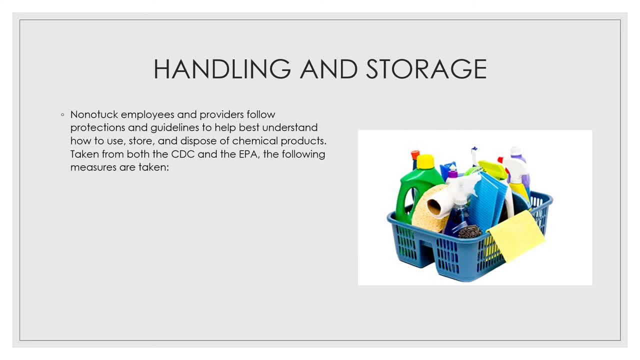 mayo. Categories and providers. follow protections and guidelines to help best understand how to use, store and dispose of chemical products, Taken from both the CDC and the EPA. Puisouo Street, Tennessee. the following measures are taken: Follow product label directions for chemical storage. 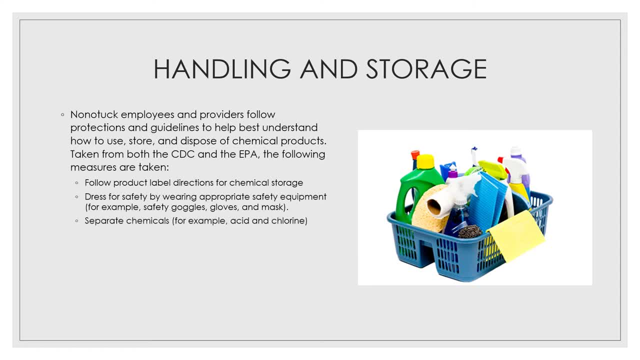 dress for safety by wearing appropriate safety equipment, such as safety goggles, gloves and masks. Separate chemicals, for example acid and chlorine, Lock chemicals up to protect people and animals. Keep chemicals dry and do not cause a reaction. by removing any chemicals that do not also have aarea ihap. 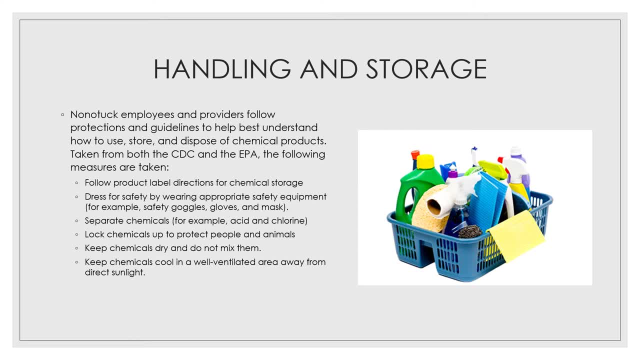 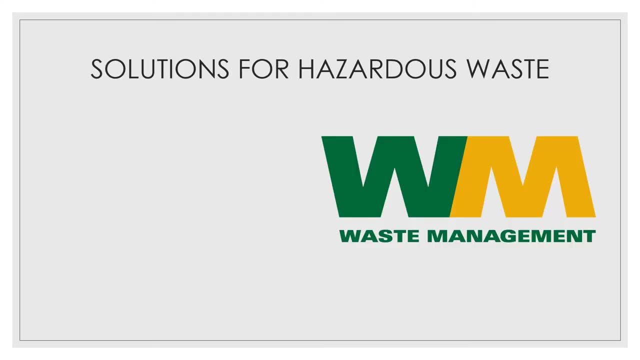 mix them, keep chemicals cool in a well-ventilated area, away from direct sunlight, and keep chemicals closed in original labeled container. Solutions for hazardous waste. Waste management has decades of experience managing these materials responsibly and can remove them with their at-your-door special collection service Or, if the service isn't available in your area. 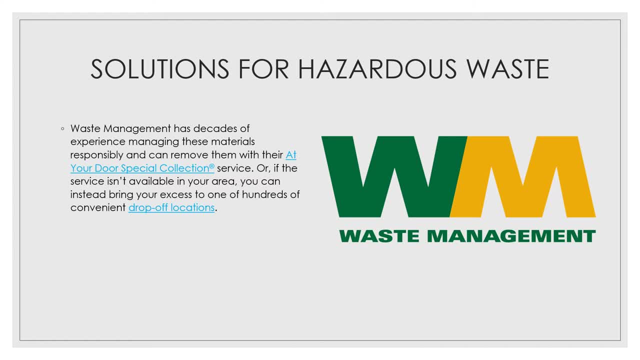 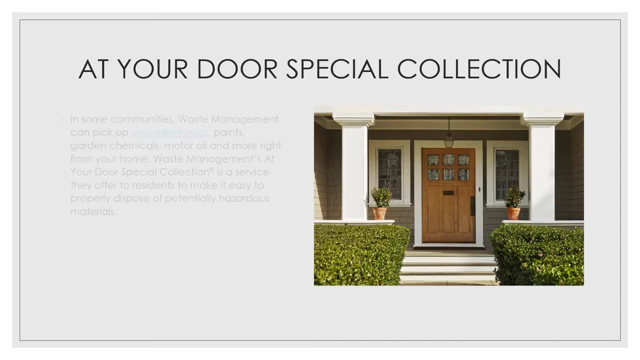 you can instead bring your excess to one of the hundreds of convenient drop-off locations. Waste management helps disposing of these potentially dangerous items not only easy but safe from your household or your business At-your-door special collection. In some communities, waste management can pick up. 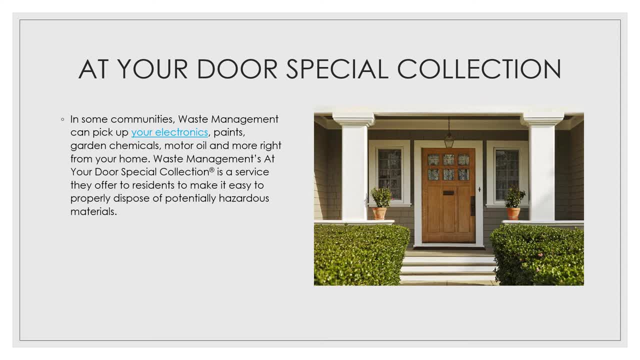 your electronics, paints, garden chemicals, motor oil and more right from your home. Waste management's at-your-door special collection is a service that they offer to residents to make it easy to properly dispose of potentially hazardous materials. To verify the at-your-door service is available in your area and schedule a collection: 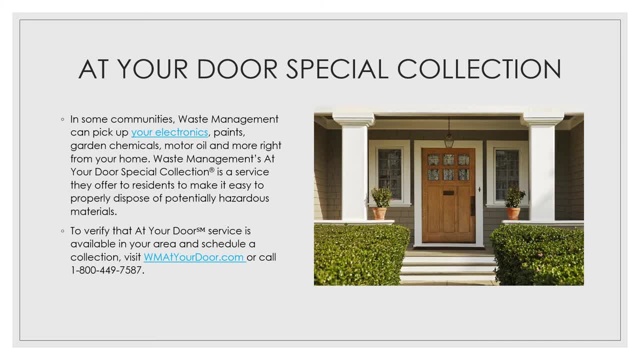 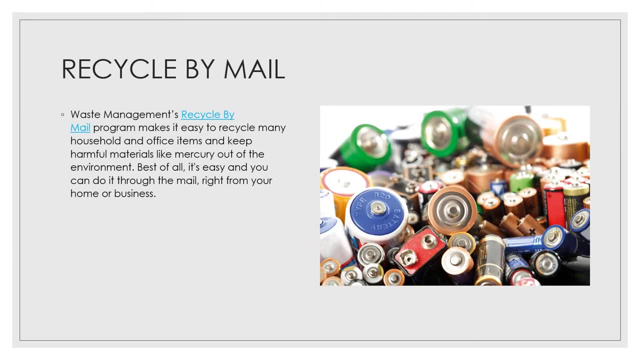 visit WMatyourdoorcom or call 1-800-449-7587.. Recycle by mail. Waste management's recycle by mail program makes it easy to recycle many household and office items and keep harmful materials like mercury out of the environment. 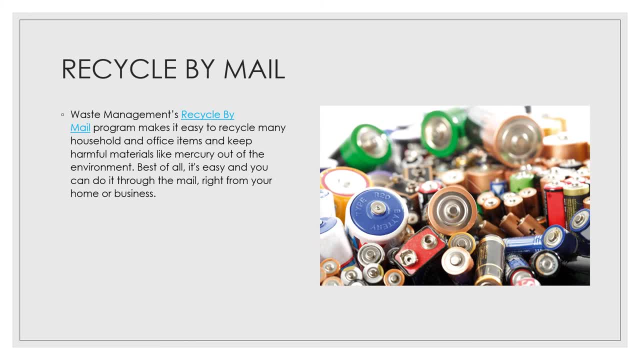 Best of all, it's easy and you can do it through the mail, right from your home or business. Waste management recycling kits come with everything you need, from the box to the return shipping label. Fill them up, send them back and they'll take care of the rest.